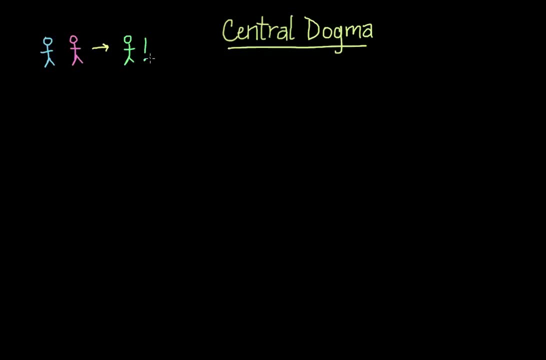 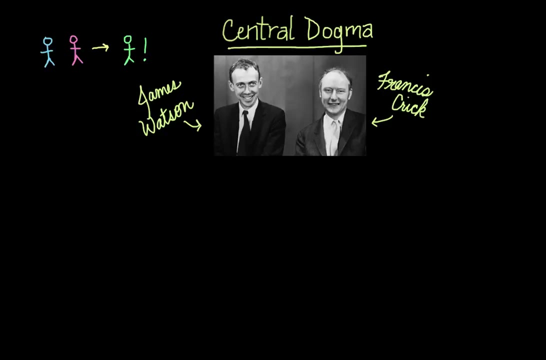 full-blown human being like you and me. So some very clever scientists- Francis Crick and James Watson, or Watson and Crick, as they're often referred to, as are credited with discovering this dogma, which they say deals with the detailed residue-by-residue transfer of sequential 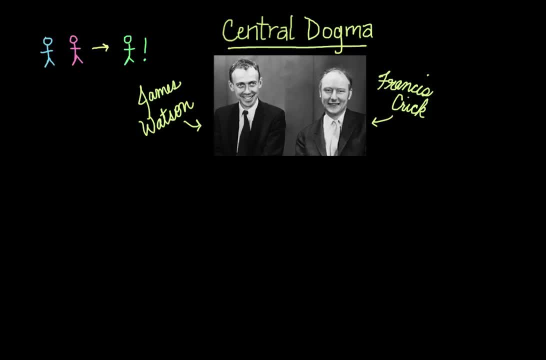 information. Or as Marshall Nirenberg, who won the Nobel Prize in Physiology and Medicine, once said: DNA makes RNA makes protein, And I think this simple explanation really just says it all. So let's explore this concept a little bit further. So we have three major players here. 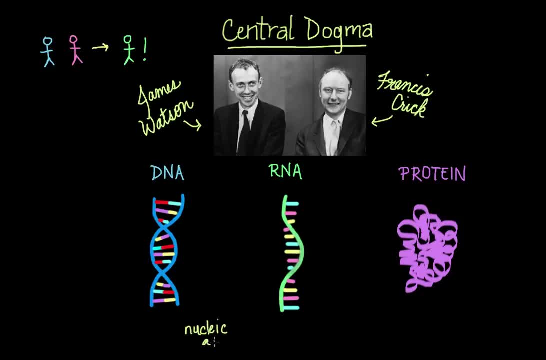 DNA and RNA. DNA are nucleic acids which are made up of nucleotides, And proteins are made up of amino acids And the information starts at the most basic level, stored as DNA, which can then be restored as DNA. when DNA copies itself in a process called replication, Then DNA can be copied into. 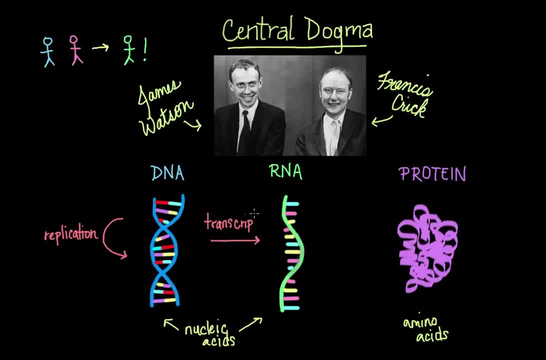 RNA in a process called transcription, And then, finally, you can use the information in RNA to synthesize a protein In a process called translation. Now, since DNA, RNA and protein are linear polymers, this means that each individual unit or monomer is only attached to at most two other units. So say, we have a monomer which is just 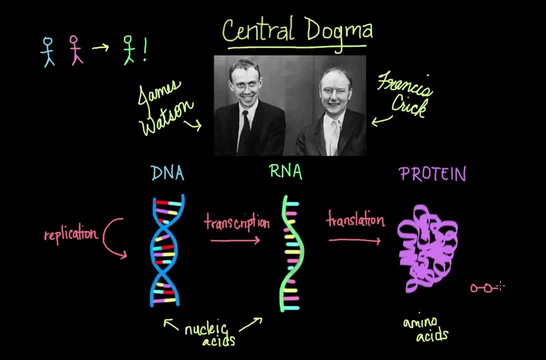 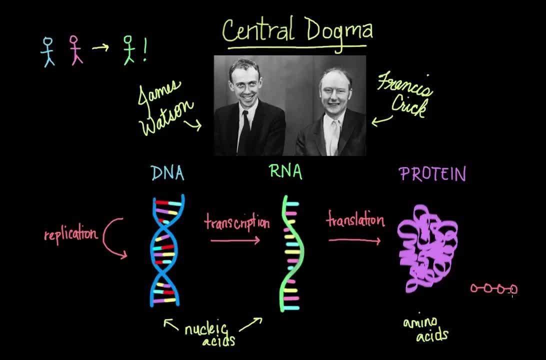 DR, Which are just amino acids all connected in a linear polymer, DR. So what does this mean? DR? This means that the specific sequence of each of these monomers effectively encodes information and that the transfer of information is faithfully preserved from DNA to RNA to. 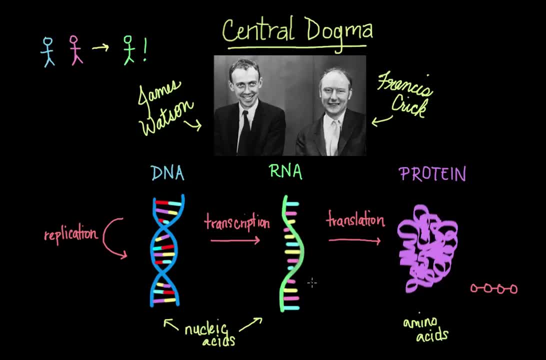 protein: DR. Each polymer sequence is used as a template for the synthesis of the next polymer, DR. You can go into any step in this sequence and determine what the corresponding polymers would look like? DR. What is the transfer of information that is prior to separation? 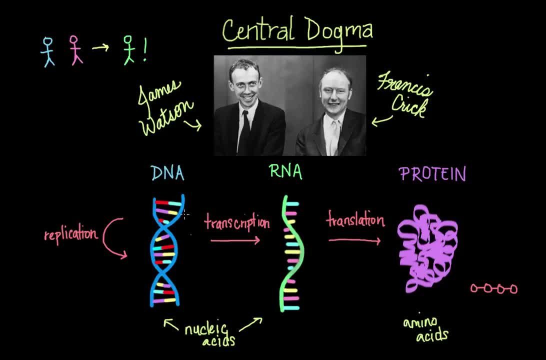 So in other words, you could take DNA and obviously figure out what the corresponding RNA would look like and then what the corresponding protein would look like. So this whole process is the central dogma. It can sometimes be a little bit tricky to keep all of these terms straight. 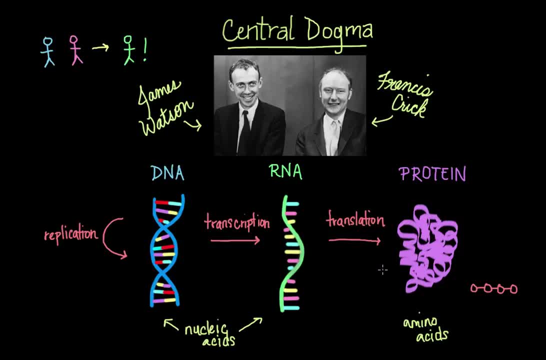 so I'll try to break it down a little bit for how I like to remember them. For DNA, I think it's pretty easy. When you go from DNA and DNA makes a copy of itself, it's called replication, because DNA is just replicating itself. 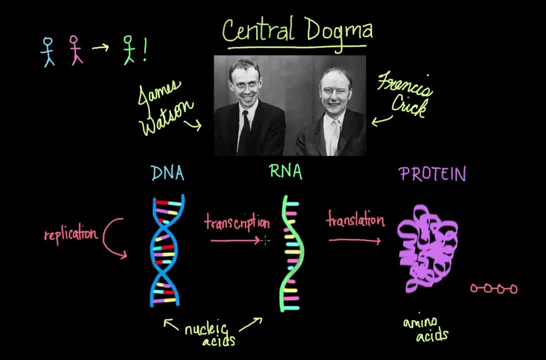 It's making the same copy of itself. Transcription and translation. on the other hand, it's kind of easy to get these two terms mixed up. One of them, obviously, is talking about DNA to RNA, whereas the other one is talking about going from RNA to protein. 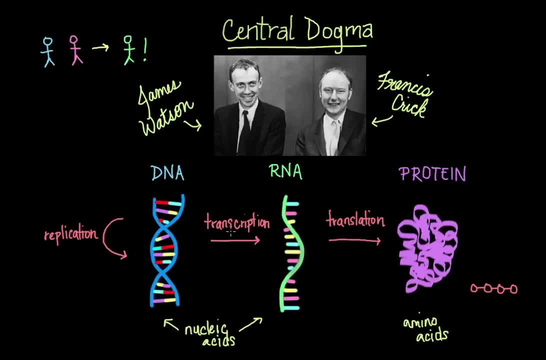 So if you look at the word transcription, it has the word script in it. So I think of it as going from one written form to another, to another kind of written form, And both use nucleic acids, So they both use this sort of alphabet, if you will. 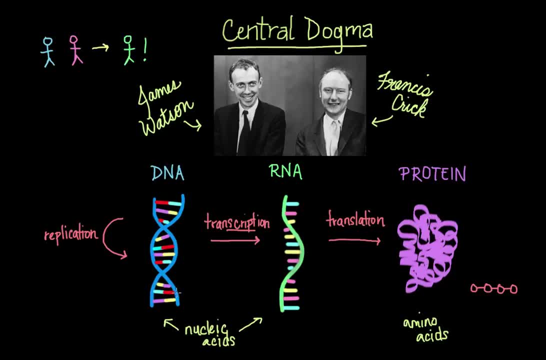 of nucleic acids, And so you're just going from one kind of alphabet to the next kind of alphabet. Translation, on the other hand, which is also the same term that we use when translating one language to another, describes going from nucleic acid to amino acid. 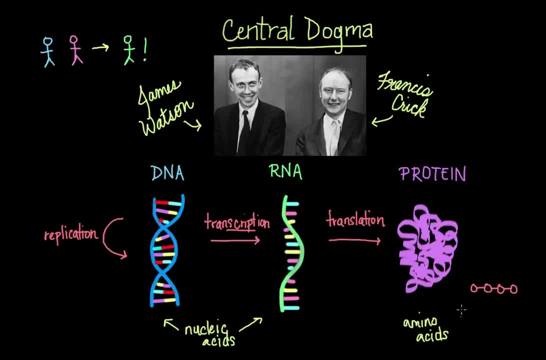 So it's like you're using one kind of language to another kind of language Because you're going from nucleic acid building blocks to amino acid building blocks. So hopefully that helps you keep these terms straight a little bit. So what did we learn about the central dogma? 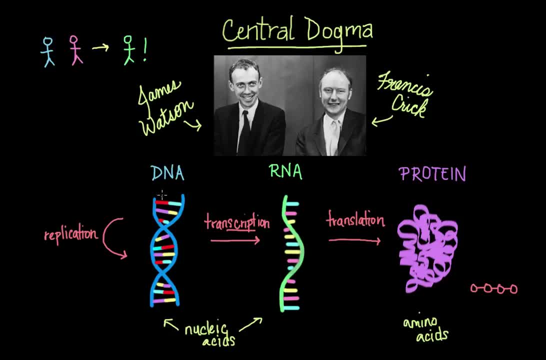 Just remember the simple statement that DNA makes RNA, which makes protein.